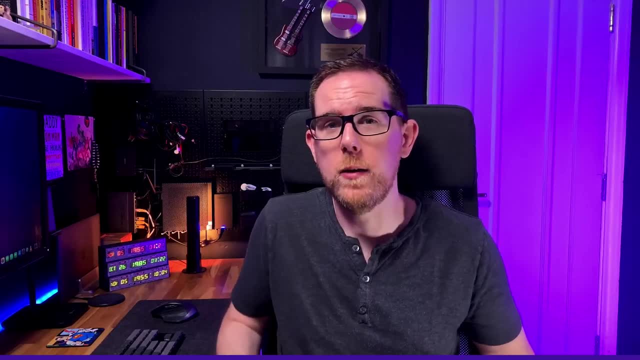 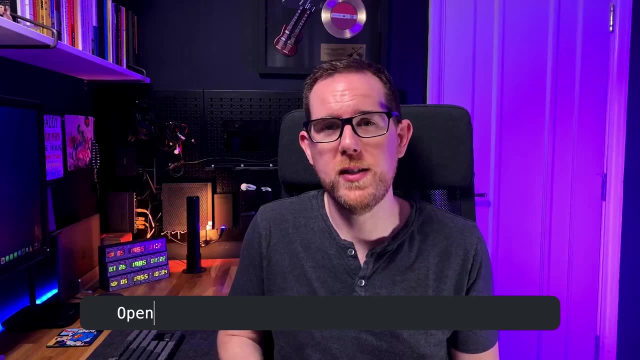 everything it does should be very closely related, so you don't end up with bloated classes. The second principle is the open- close principle. Now, this principle states that your code should be open to extension, but closed to extension. This means that your code should be open to extension. 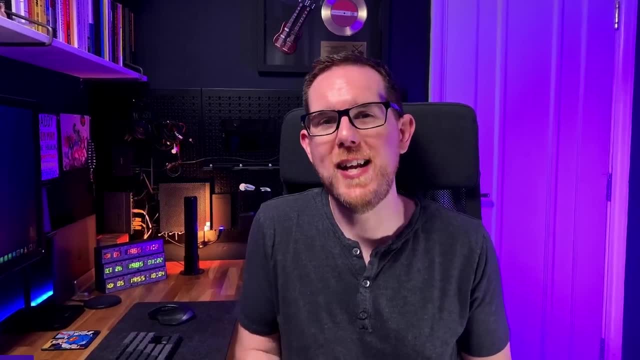 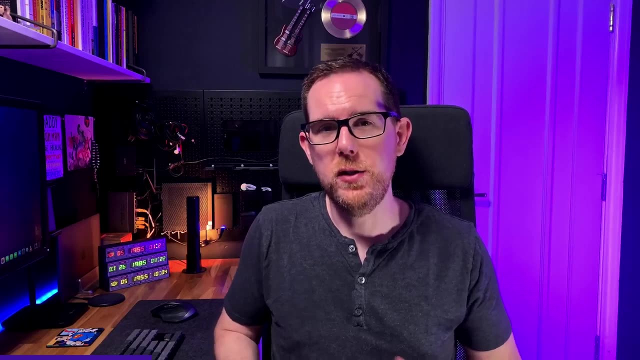 but closed to modification. If you need to add some additional functionality to your application, then you shouldn't be editing the existing classes or methods to do that. After all, you have spent ages writing unit tests for all of those methods and therefore any changes you make now would cause. 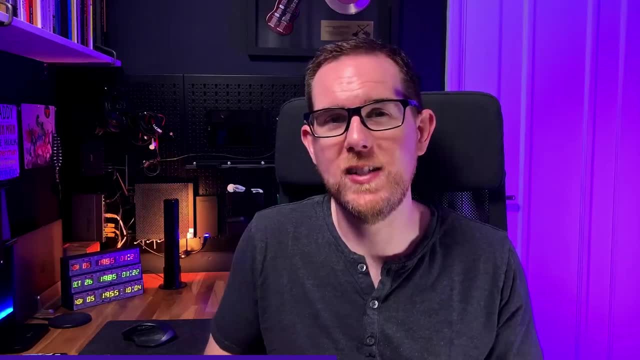 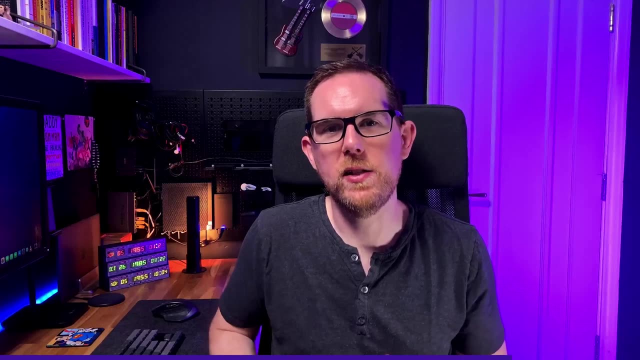 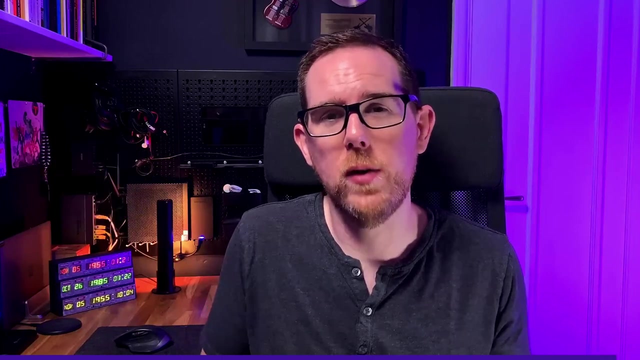 them to break. On top of that, adding in additional functionality to existing methods may cause unexpected consequences wherever you end up calling that method from. So how do you go about adding additional functionality without changing the existing methods or classes? For these examples, you'll need to check with your language documentation to see which ones are available to. 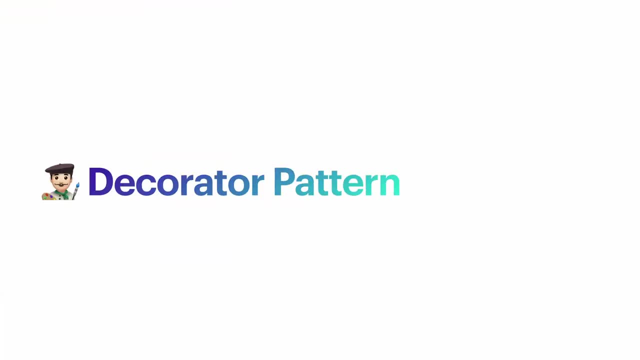 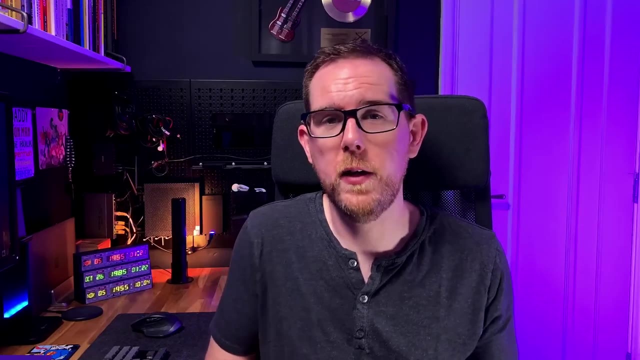 you. One way to achieve this is to use the decorator pattern. If you need to add some additional functionality, either before or after your existing code, then this is one way to do that. Instead of modifying the code, we create a new class that implements the same interface. 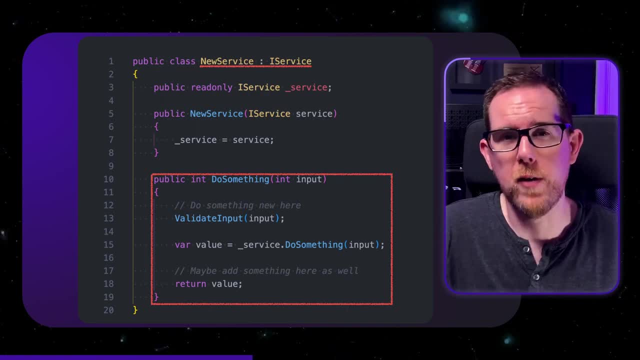 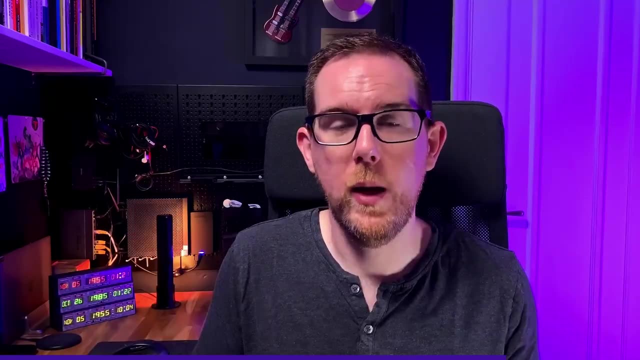 We can then call this new method without affecting the other code in our application. The benefit of this approach is that you can use dependency injection at runtime to be able to control when this new class is used. However, you can only use this approach if the method you want to extend is both public and included in the interface. 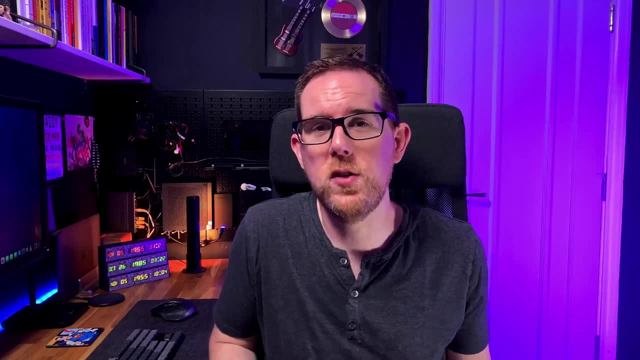 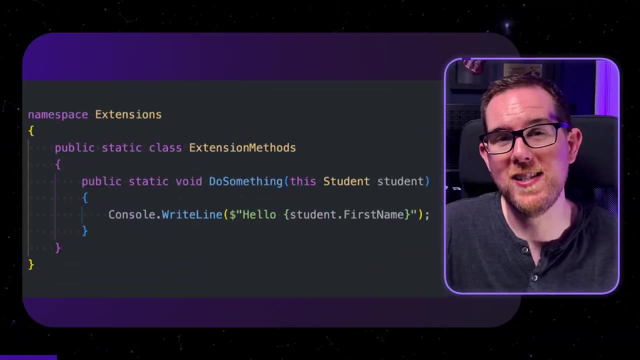 Another great option is to use extension methods. Now, extension methods can be used in both C, sharp and Kotlin, as well as a few other languages. An extension method allows you to add a method to an existing class without actually having to change that file, Provided that you have the namespace. 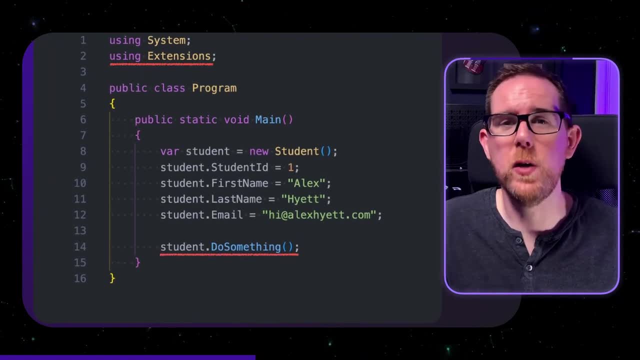 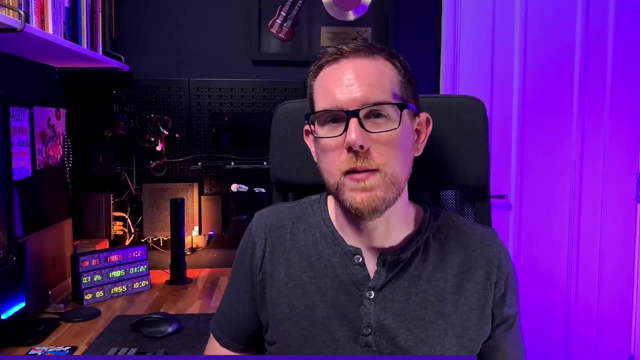 for your extension imported. you can then use the method in the same way you would do if that method was part of the original class. The only downside of using extension methods is that, unlike the new method, you can't switch at runtime when this code is used. There are many different ways that. 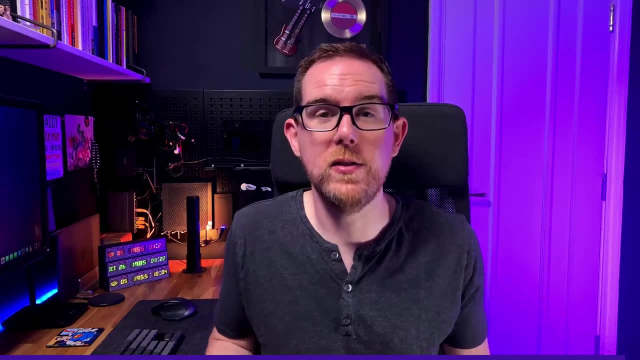 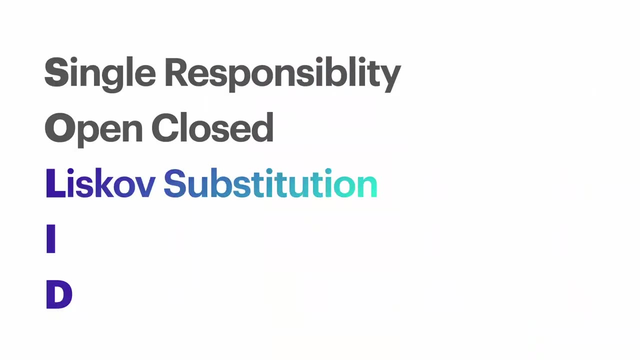 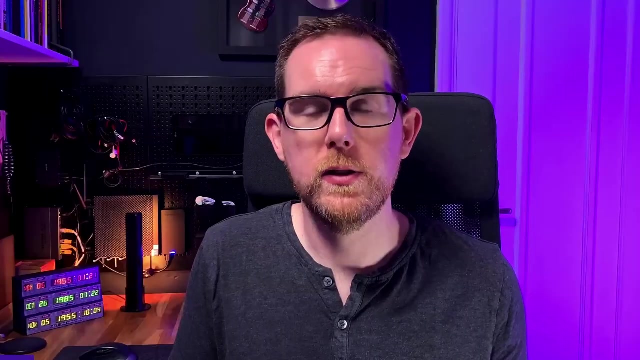 you can extend the functionality of your application without having to change the existing code, such as using inheritance or attributes. The next principle is the Liskov substitution principle. Now, this principle is a little harder to understand. It states that a child class should be able to do everything that a parent class can. So let's say we have an actual parent class and 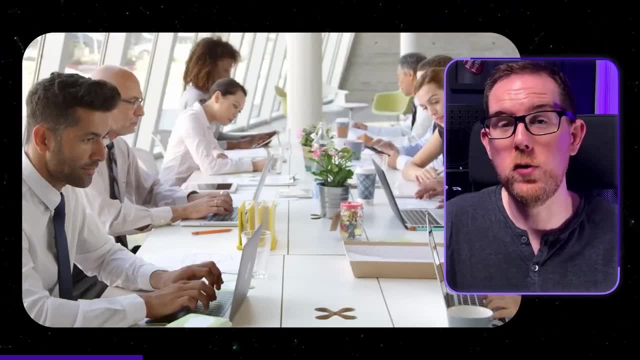 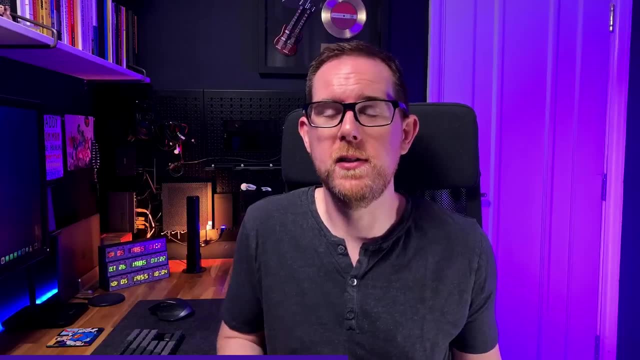 it might be able to do things such as eat, sleep, go to work and make dinner. Then we have a child class that is inherited from that parent class. Now, obviously, as a child, there's some things they can't do, such as make dinner and go to work. This would therefore break the Liskov substitution. 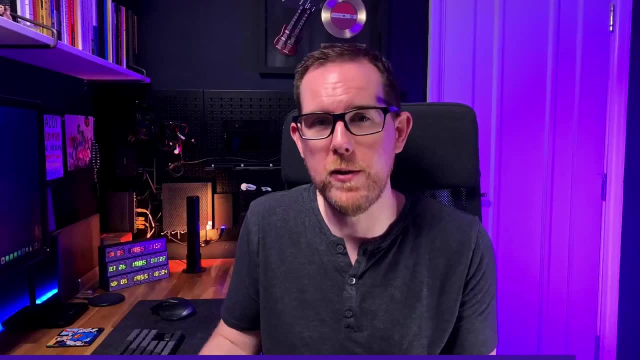 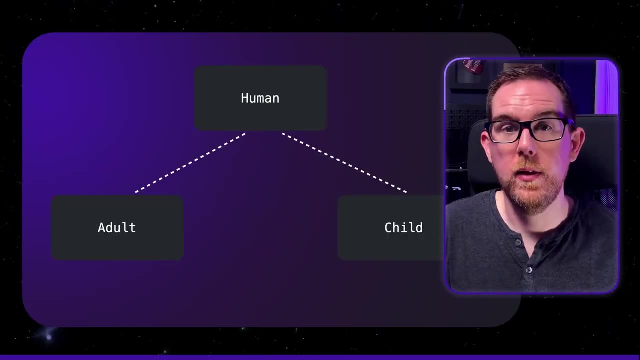 principle because we can't use the child wherever we've used the parent in our code. To fix this, we'd have to create a human class and then have an adult and child class that would inherit from that instead. The next principle is the interface segregation principle. Now, interfaces provide a 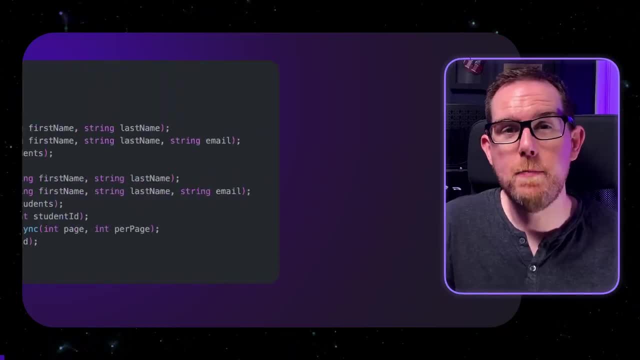 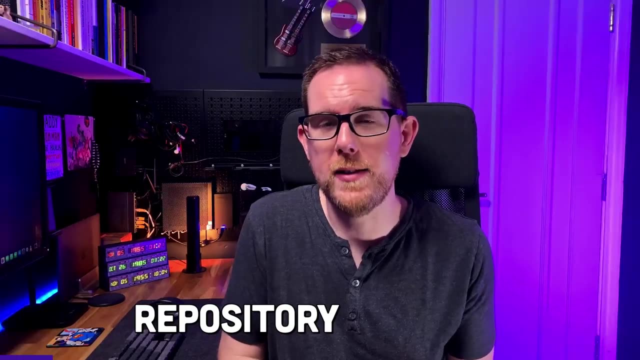 contract that your classes need to implement. If you have particularly bulky interfaces, then your classes will be forced to implement methods they might not end up using. If you've ever used a repository pattern, you might have come across this before. With this pattern, you end up writing an. 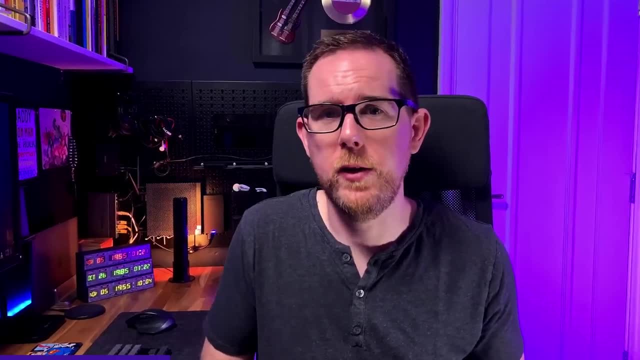 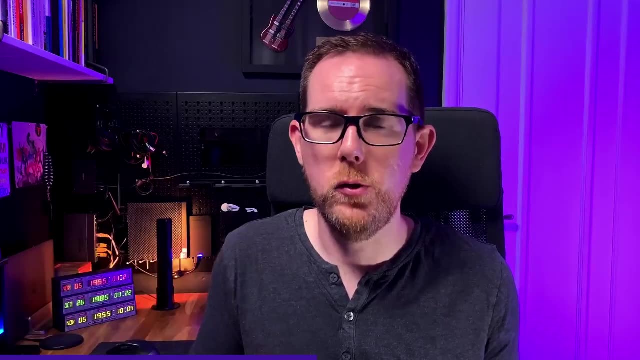 interface that looks a bit like this. Now, every time you end up using this interface, you need to write an implementation for each of those methods, even if you don't plan on using them. If you didn't want to implement any of these methods, you could, of course, throw a not implemented exception, but 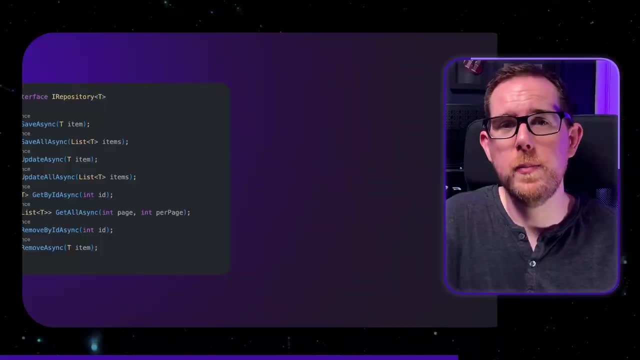 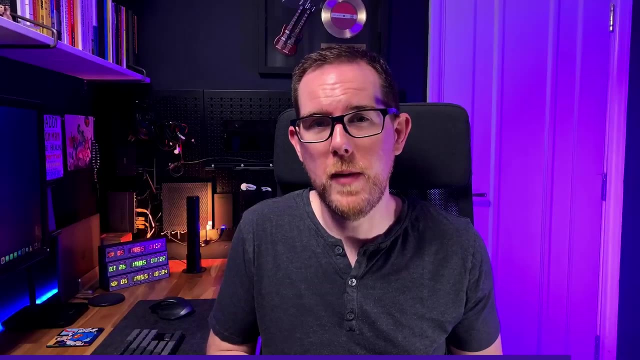 that would then break the Liskov substitution principle as well. To overcome this, you can split the methods into different interfaces. You might have one for writing, one for reading and one for deleting. When you do need to use all of the different methods, you 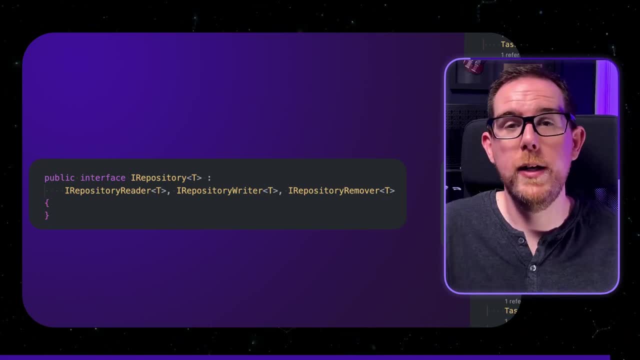 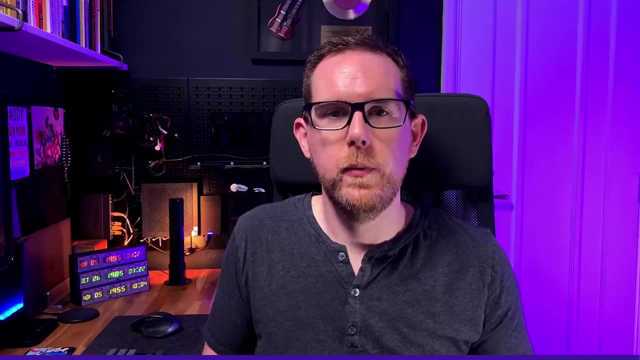 could always create a main interface that inherits from all the others. This way, you only need to implement the methods that you're actually going to use, and you don't need to worry about calling some code that hasn't been implemented yet. The last principle of SOLID is dependency inversion. 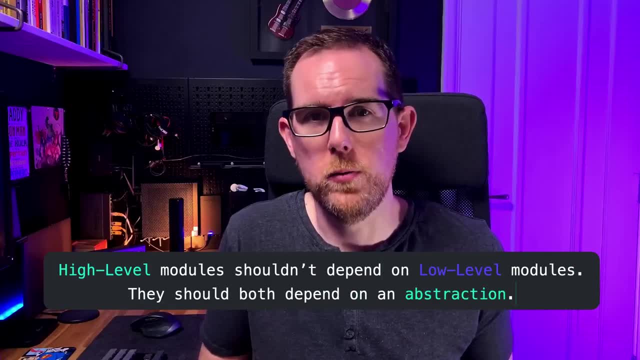 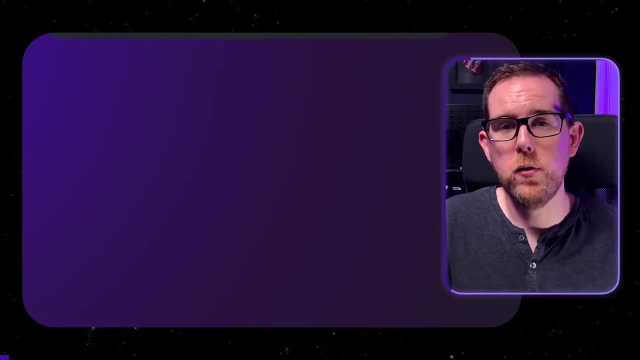 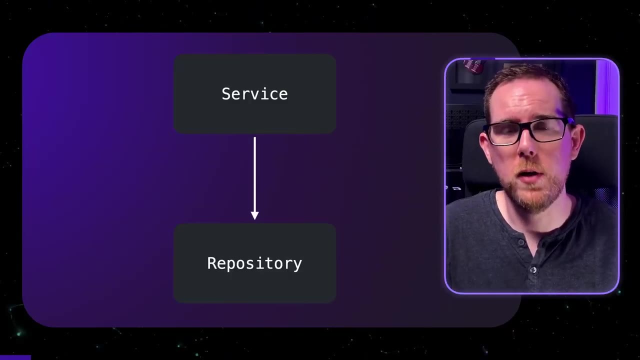 which states that high level modules shouldn't depend on low level modules. They should both depend on an abstraction. For example, if you had a service class and you wanted to save something to a database, you could create an instance of the repository class dot directly inside your service, But now your service is dependent on a lower level component. 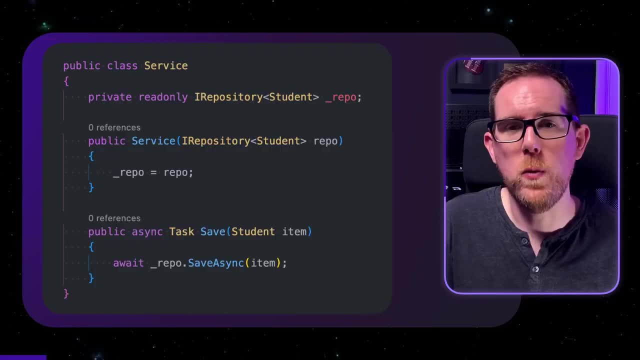 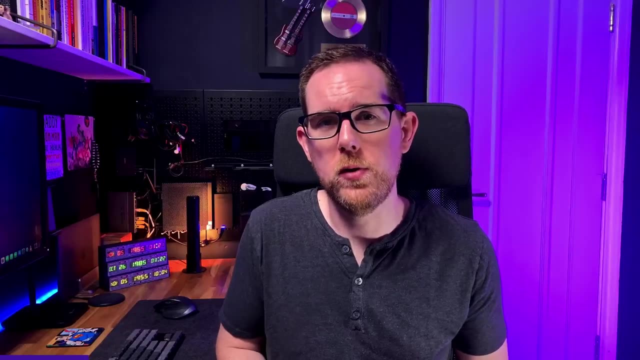 To overcome this, we create an interface for our repository and then we inject an instance of the repository into that class via the constructor. Now, both the high level and low level modules depend on an abstraction, which, in this case, is the interface. The service doesn't need to know which.